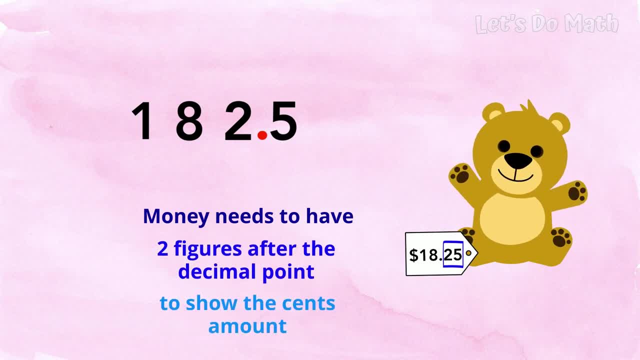 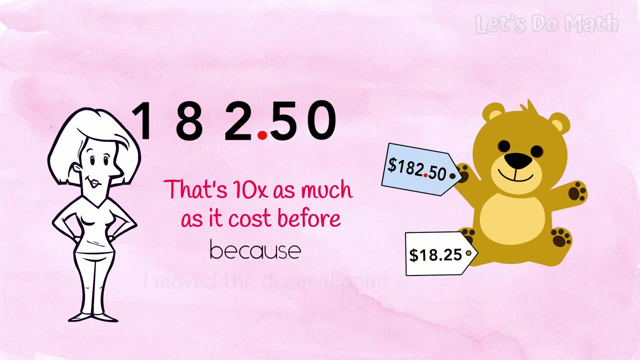 Money needs to have TWO figures after the decimal point to show the cents amount. So we put in a zero And now you can see that the teddy costs That's 10 times as much as it cost before, because I moved the decimal point one place to the right. 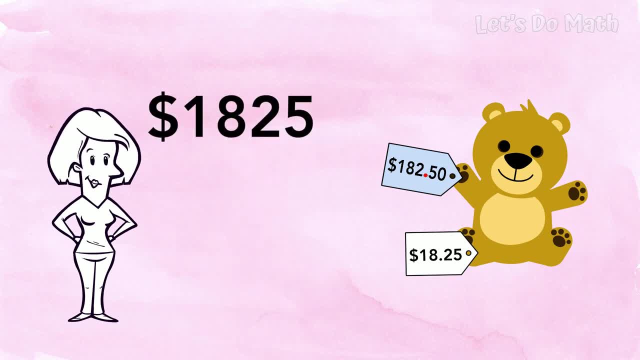 And what if I do this? Wow, that's a lot for a stuffy. These 4 digits and no decimal means. this is one expensive bear. Of course we should put the decimal point and two zeros to write the money amount properly. 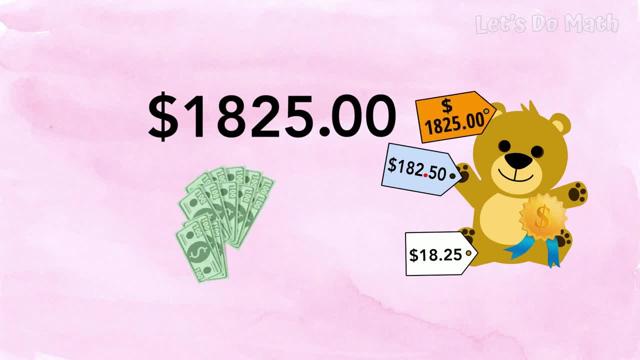 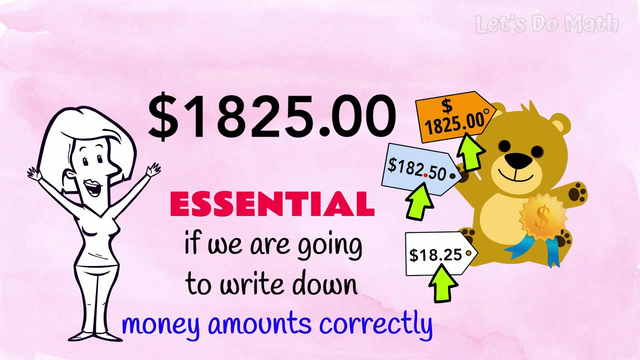 So the bear now costs $1,825. You can see the position of the decimal point is really important. It's a big part of understanding place value and it's essential if we're going to write down money amounts correctly, Paying attention to place value. 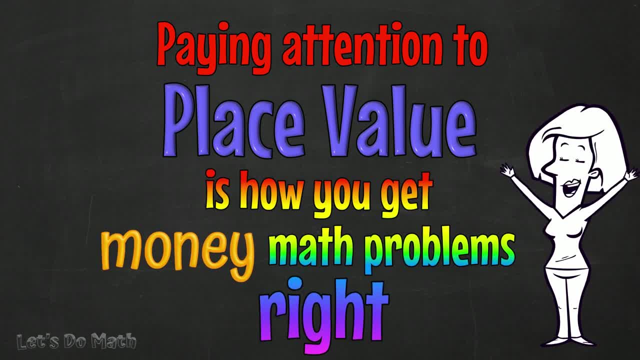 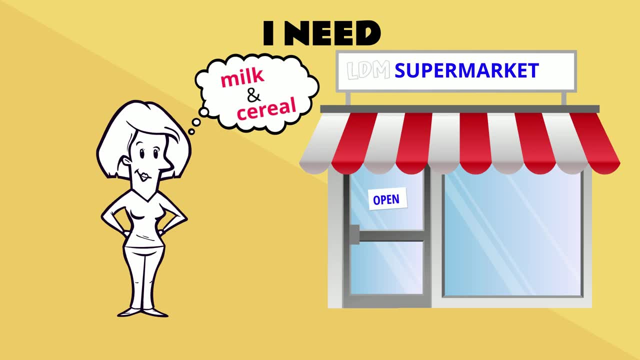 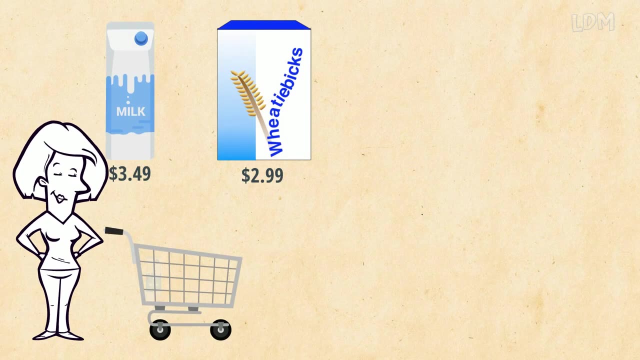 is how you get money. math problems right. I'll show you what I mean with a trip to the shop. I need milk and cereal for breakfast. I've got $10 in my pocket. I get a 2 litre carton of milk and some Weetabix. 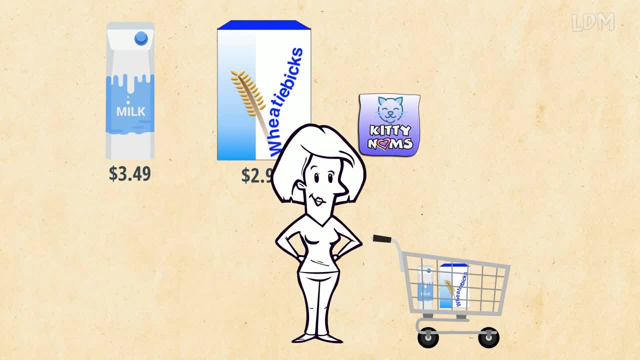 I walk up the pet food aisle and I pick up a bag of treats for my cat, Jambo. I didn't plan to buy anything for him, but it's $0.95 and he likes these things a lot. And then I see this fabulous. 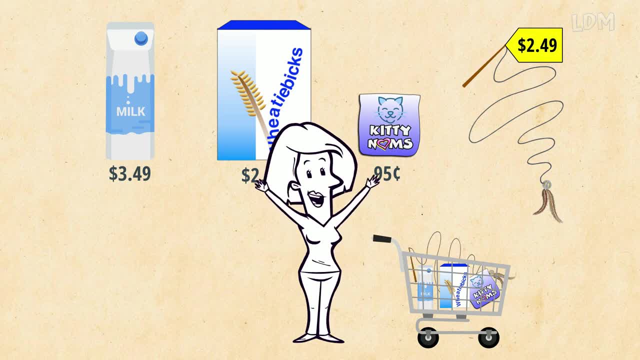 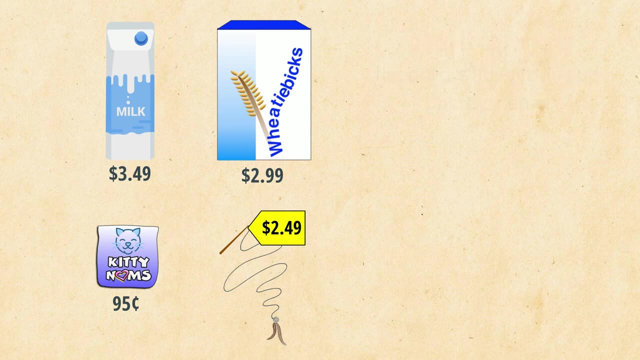 fishing for cats toy. He'll love this. Uh oh, I hope I've got enough. Luckily I have a notepad and pen with me so I can check before I get to the cashier. To add it up properly, the dollars have to line up and the cents. 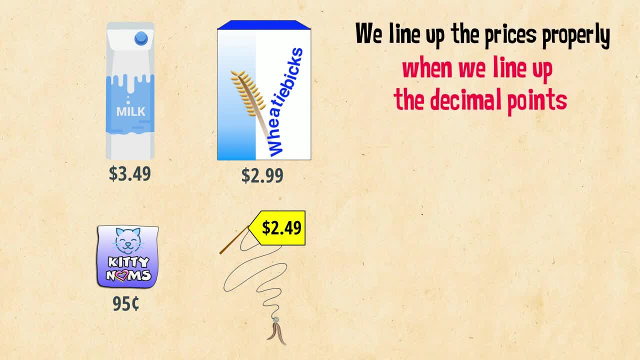 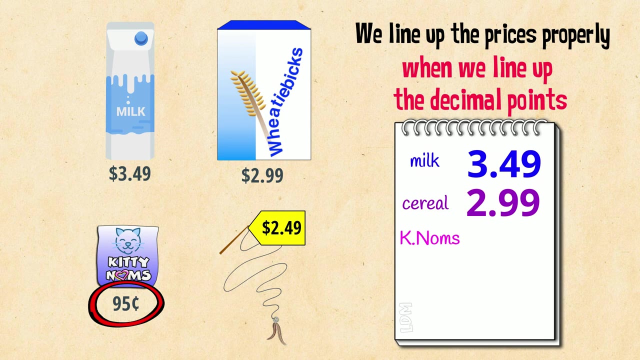 We line up the prices properly when we line up the decimal points. Let's set it up: The milk is $3.49, Weetabix is $2.99. Kitty noms are $0.95 and we show that as $0.95. 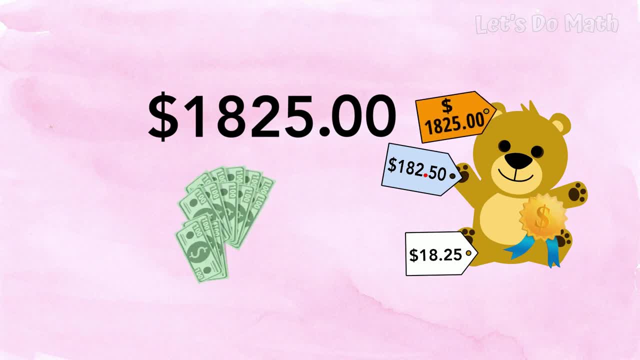 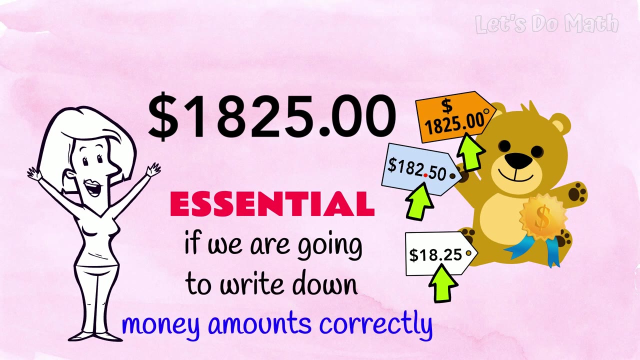 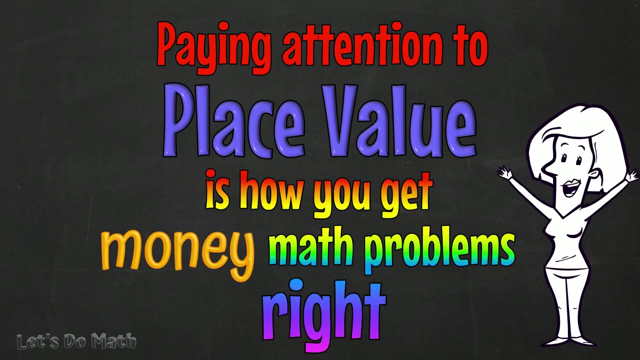 So the bear now costs. You can see the position of the decimal point is really important. It's a big part of understanding place value And it's essential if we're going to write down money amounts correctly. Paying attention to place value is how you get money. math problems right. 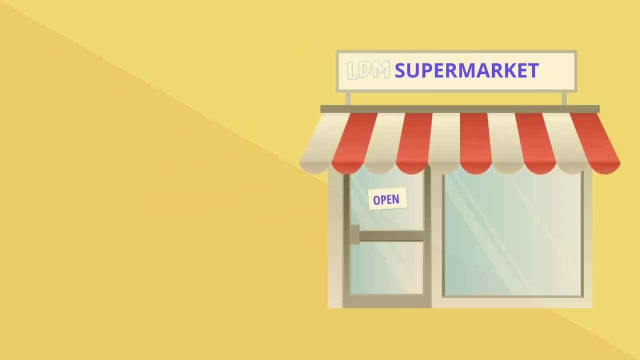 I'll show you what I mean with a trip to the shop. I need milk and cereal for breakfast. I've got $10 in my pocket. I get a 2 litre carton of milk and some Weetabix. I walk up the pet food aisle. 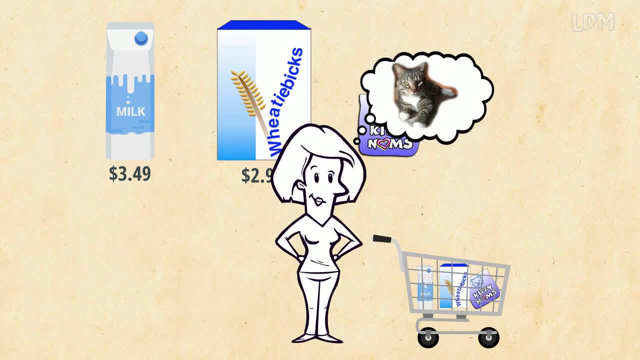 and I pick up a bag of treats for my cat, Jambo. I didn't plan to buy anything for him, but it's $0.95 and he likes these things a lot. And then I see this fabulous fishing for cats toy. He'll love this. 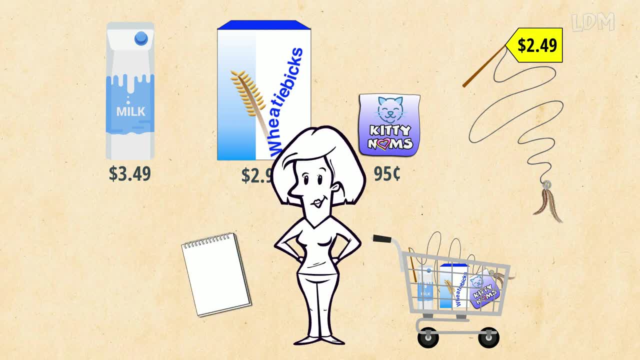 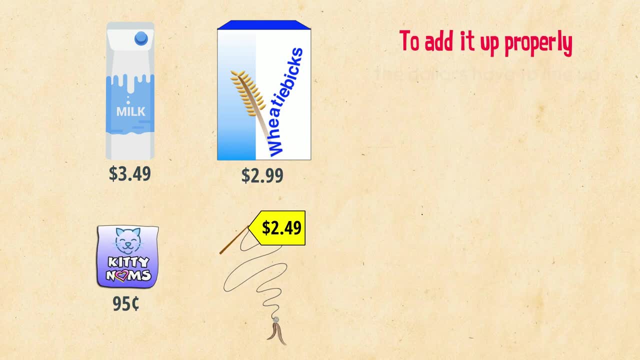 Uh oh, I hope I've got enough. Luckily I have a notepad and pen with me so I can check before I get to the cashier. To add it up properly: the dollars have to line up and the cents. We line up the prices properly. 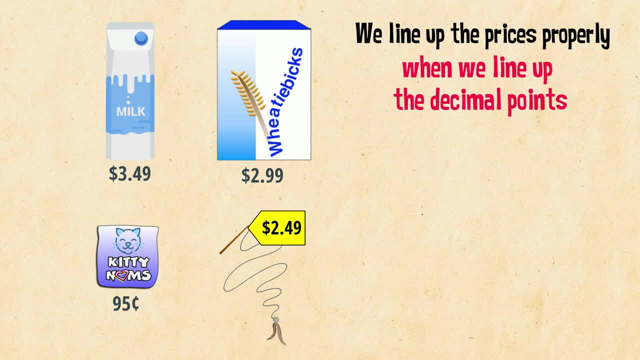 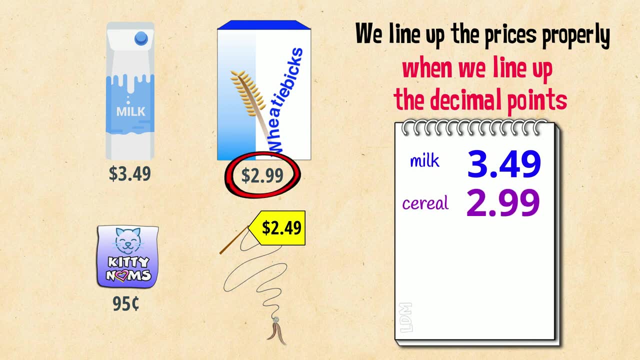 when we line up the decimal points. Let's set it up: The milk is $3.49, Weetabix is $2.99, Kitty Noms are $0.95 and we show that as $0.95, and Fishing for Cats is $2.49. 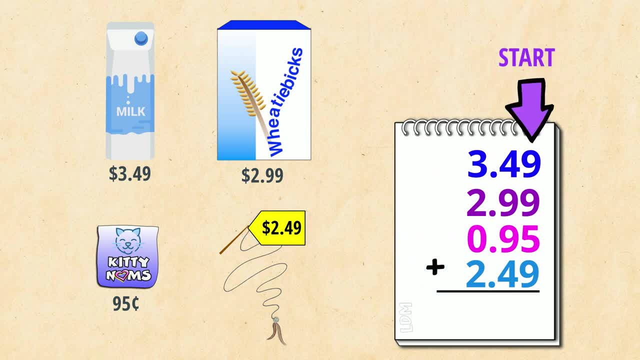 As with all addition, problems start in the RIGHT HAND COLUMN. I've got 3 9s here, That's 27.. Plus 5 is 32.. Next, I've got 2 9s, That's 18.. Plus 4 is 22.. 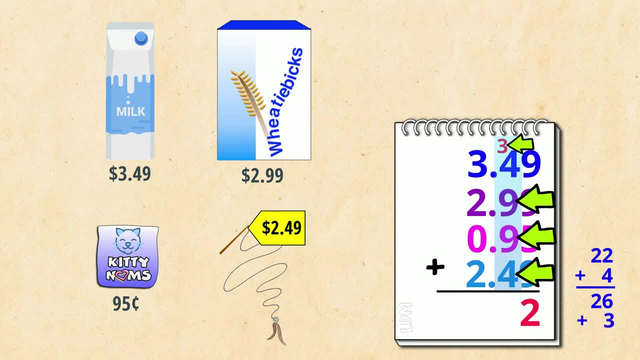 Plus another 4 is 26.. And this 3 is 29.. Now we put in the decimal point And in the dollars column We've got 2 and 3 is 5.. Plus 2 is 7.. Plus this 2 is 9..